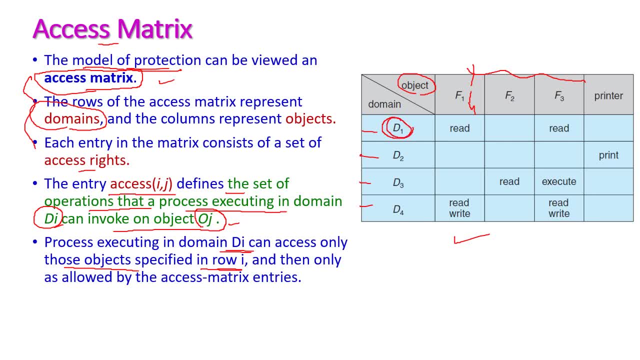 Okay, for example, suppose I am going to access this domain 1, then the domain 1 can access the file 1 and file 3 and that to the readout, So it can perform only the readout operations on file 1 and file 3.. 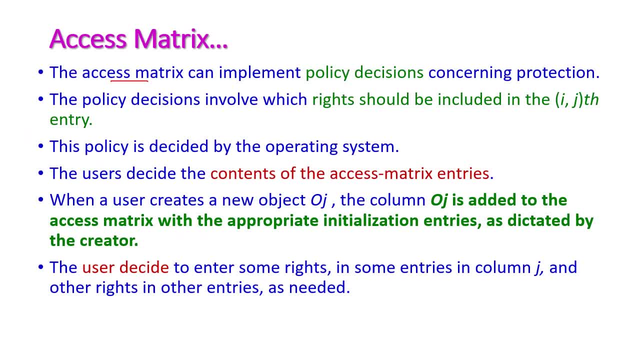 Okay, access matrix can implement the policy decisions concerning the protection. That is, we need to protect all the resources. which user can access which particular resource? Okay, that will be decided by access matrix And the policy decisions involved. the rights should be included. 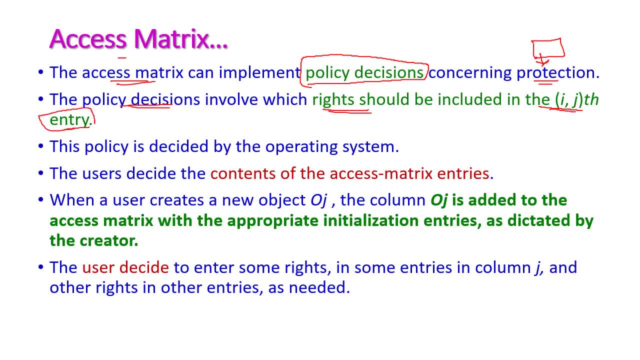 In i jth entry in the access matrix Right and this policy will be decided by operating system. Then what will the user will do? The user will decide content of access matrix entries. Once the user create a new object, immediately a column will be included in the access matrix. 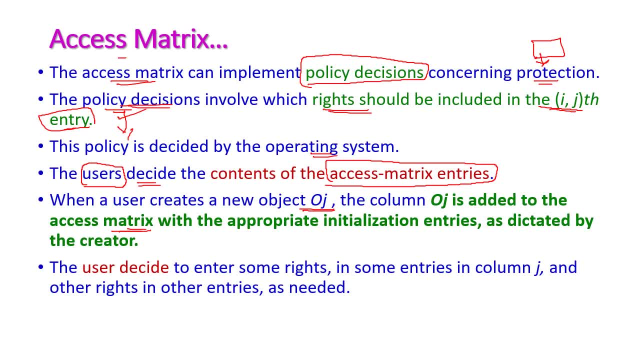 Okay, to decide which particular access will be given for this particular object And dictated by the creator, which are dictated by the creator. So that is in the access matrix. if we create a new object immediately one column will be added in the access matrix. 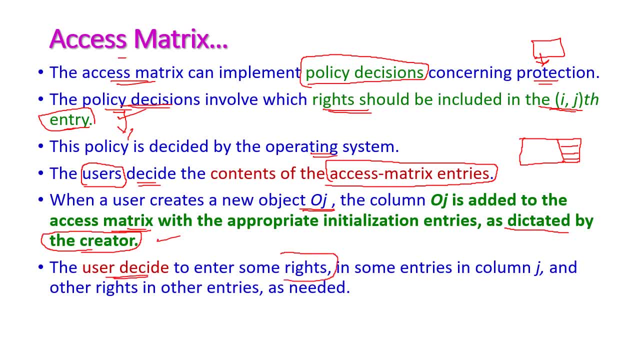 And the user can decide to enter some rights for this particular object. It can be: read for one domain, write for another domain, execute for another domain likewise. And next let us see the access matrix. Okay, So let us see the access matrix with domains as objects. 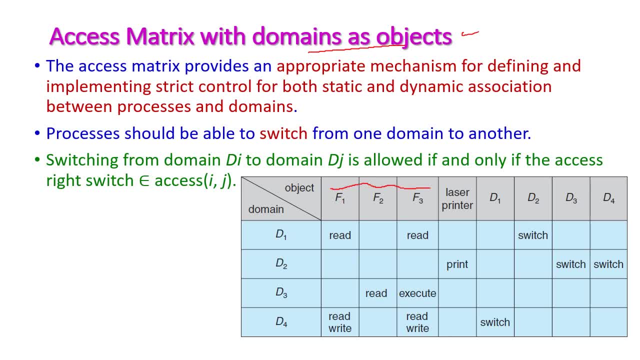 Okay, previously we are having only objects, But now we have to include domains as objects in the access matrix. Here, the access matrix provides an appropriate mechanism for defining and implementing strict control for both static and dynamic association between the process and domains. 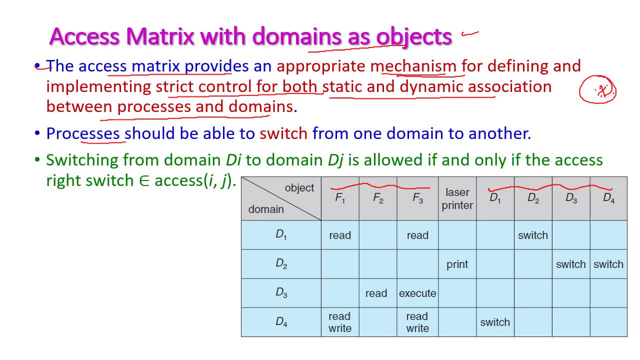 This is important here And here the process should be able To switch from one domain to another domain. That should be defined in the access matrix itself. That means the switching from domain I to domain J. That is a process wanted to switch from domain I to domain J.